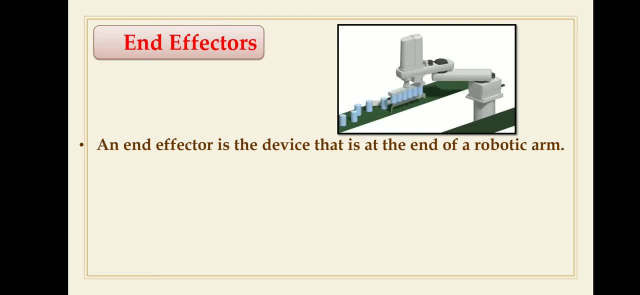 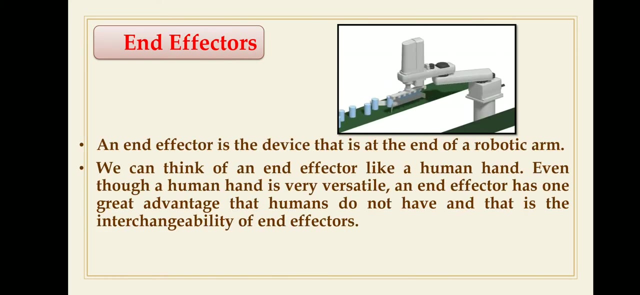 object, or to pick the object from one location and placed to another location means the end-effector is the gripper or end of arm tooling attached to the wrist of manipulator to accomplish the desired task. We can think of an end-effector like human hand, even though human hand is very versatile. 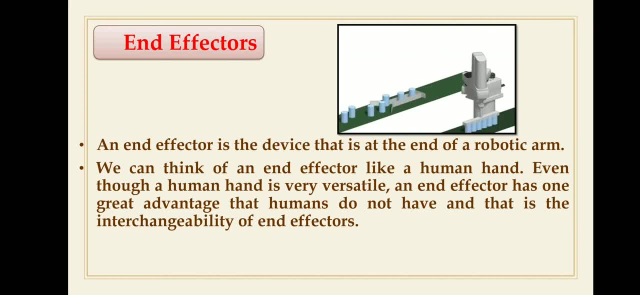 Means. one more important characteristics of end-effector is the interchangeability. Means human hand doesn't have interchangeability characteristics. That's why the important characteristics of end-effector is the interchangeability. you can easily change the end-effector as per your task. This is the important characteristics of end-effector. then the special tooling for robot that 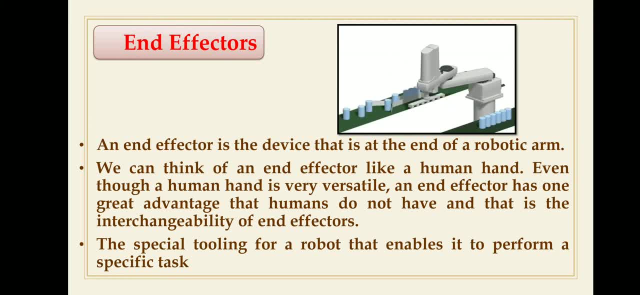 Enables it to perform a specific task. So there are different types of end-effector according to working principle and construction of end-effector, There are different types of end-effector, or end-effector is the important basic component of industrial robot. so next, different types of end-effector. 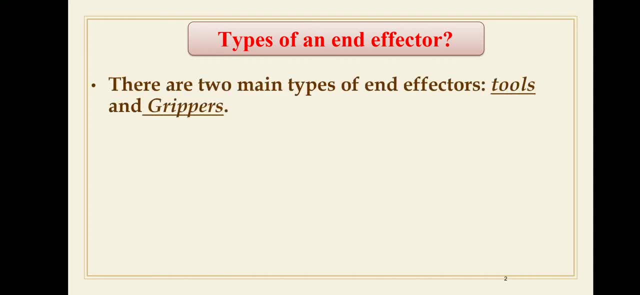 So there are two main types of end-effector: tools and gripper. These are the two main types of Grippers or end-effector. so first type is the tool, The function of tool to perform a processes like spot welding, spray painting. so in case of spot welding, 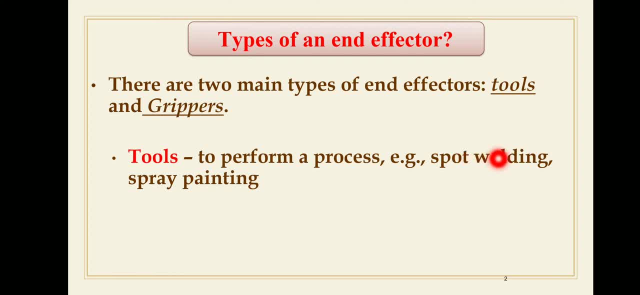 Welding gun act as an end effector means you can directly replace the end-effector. means welding gun directly attached to wrist joint for performing spot welding operation. in case of spray painting, spray painting gun act as a end effector. and another type of end effector is the gripper. the basic function of gripper to 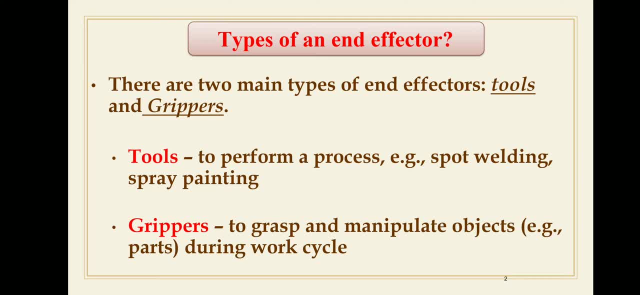 grasp and manipulate the object or part during work cycle. this is the simply function of gripper. so in that classification of end effector there are different or different types of or different classification points. so first point is the according to type of grasping modality, there are three. 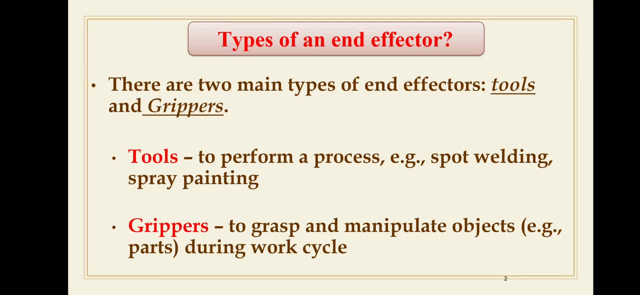 different types of end effector. first is the mechanical fingers- special tool or universal fingers. then second type, according to number of gripper mounted on wrist: single gripper mounted on wrist, multiple gripper mounted on wrist. then third type or third classification point, according to modes of gripping internal. 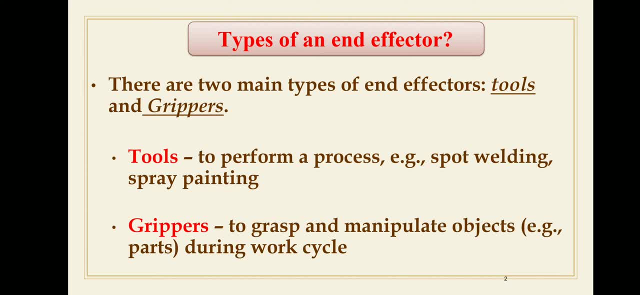 gripping and external gripping. then according to number of degrees of freedom: one degrees of freedom, 2 degrees of freedom and, last classification point, according to source of power. okay, there are three different types of end effector according to source of power: pneumatic grippers, hydraulic grippers. 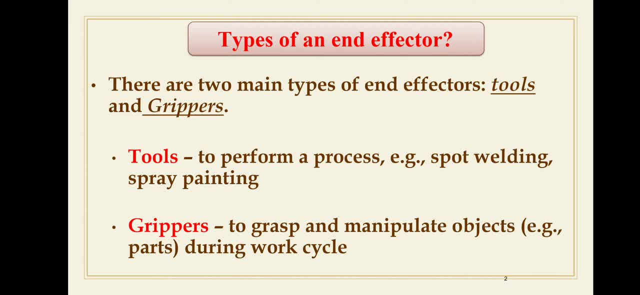 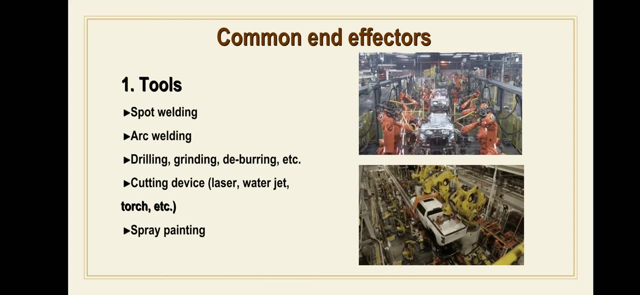 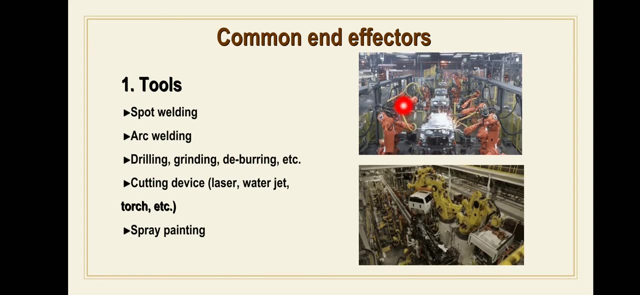 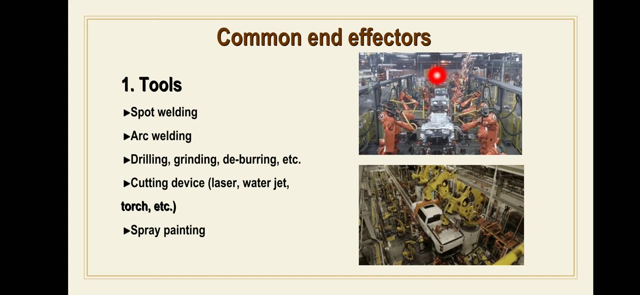 and electric grippers. so first, common types of end effectors. so first is the tool. so two animation, this is the first animation, and second, animation to animation shows the working principle of common tools. so in that first animation, spot welding or welding operation performed by industrial robot. so in this, 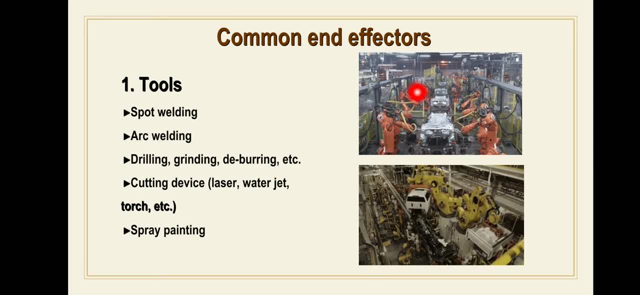 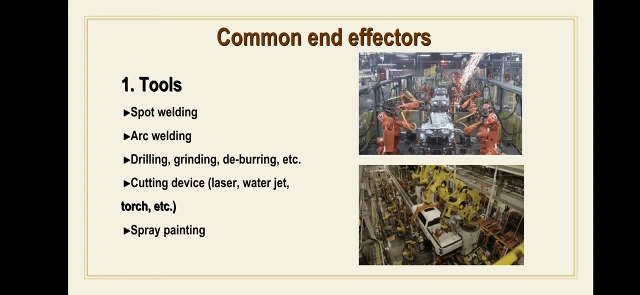 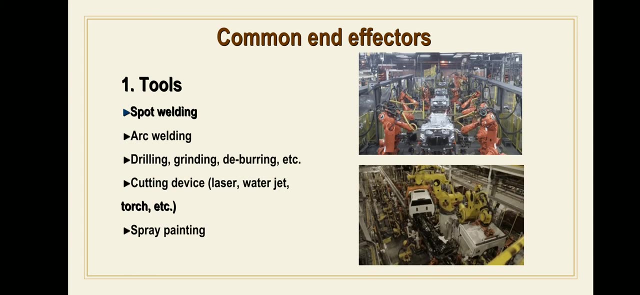 particular case, welding gun act as a end effector, or welding gun directly connect to wrist joint to perform welding operation. so first tool is the welding gun. okay, or spot welding operation perform with the help of welding gun. then arc welding means tools act as a end effector in this particular 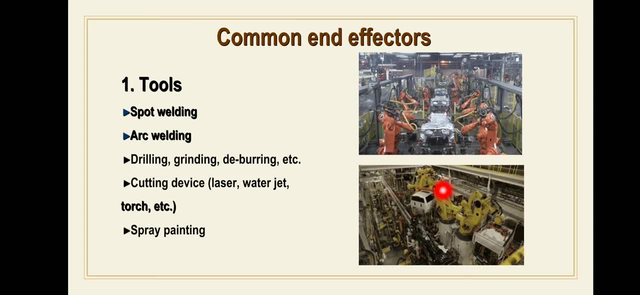 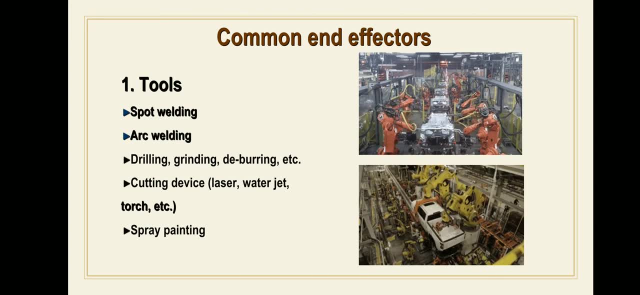 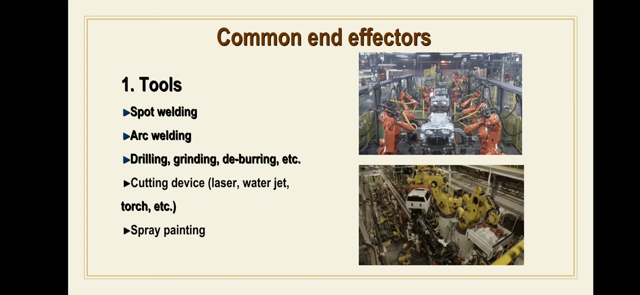 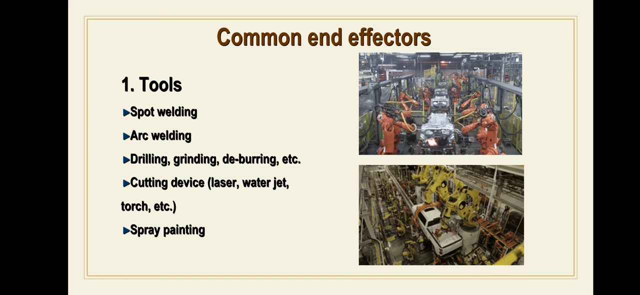 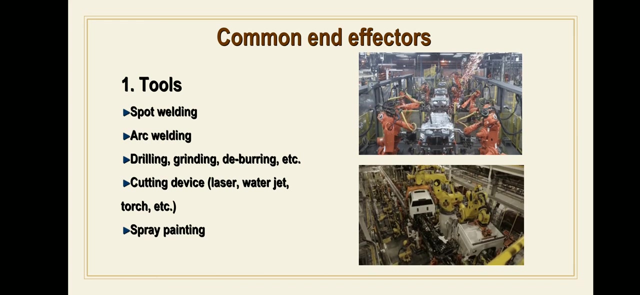 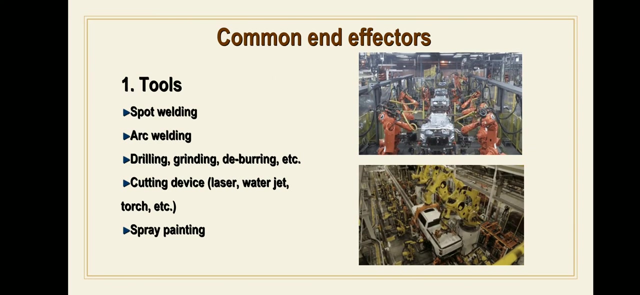 case. in that second case it shows assembly or rotation. Roman Korea machine metal metal tang, magnet, rod, accurate Arm lathe, Guy 360 et different types of mechanical end effectors to perform assembly task. okay, to perform spray painting application. then second type is the grippers. so 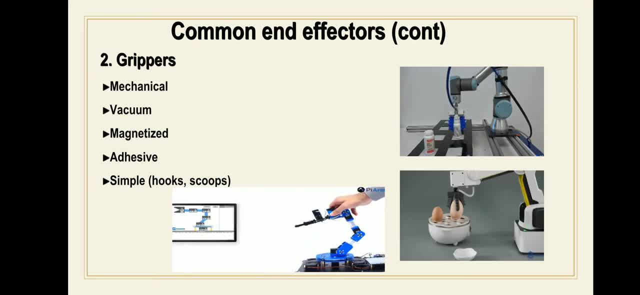 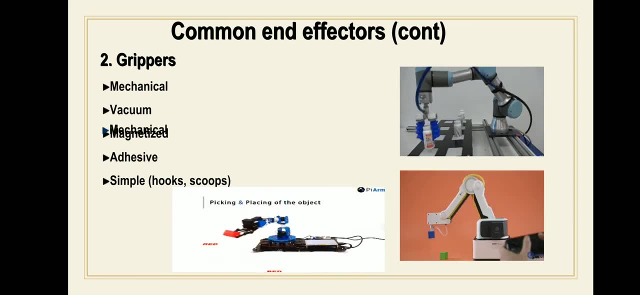 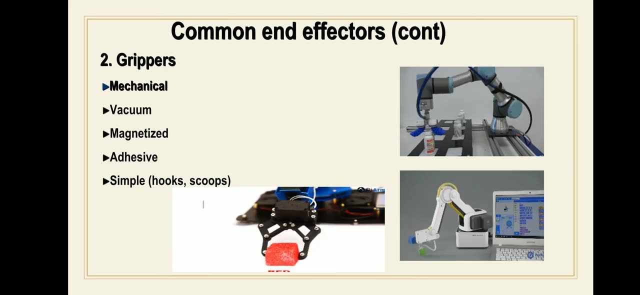 common and defective grippers. there are different types of gripper according to construction and working. there are five types of grippers. so first gripper is the mechanical gripper. means use of different mechanisms and different kinematic linkages to perform grasping- okay to grasping- operation, then vacuum. 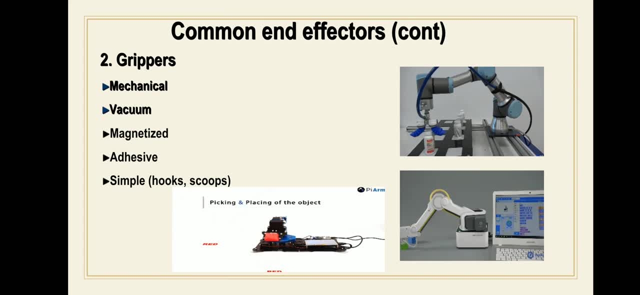 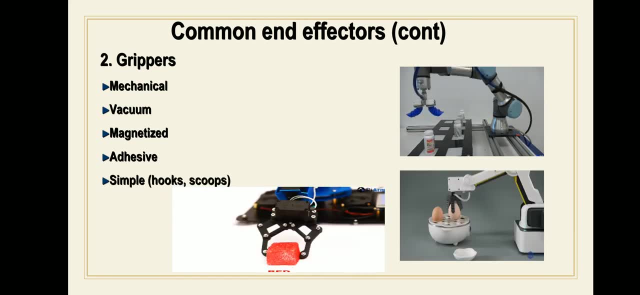 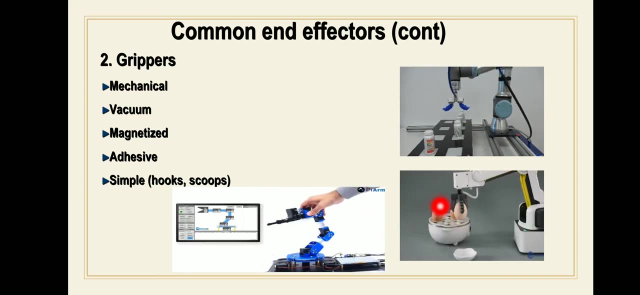 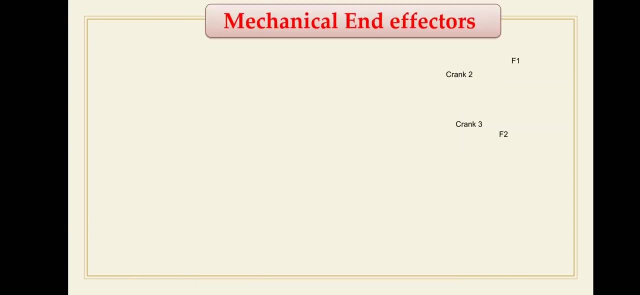 gripper: use of pneumatic principle for grasping purpose, then magnetized adhesive and simple hook. these are the five different types of grippers used in industrial robot. so this all animation shows the exactly working principle of grippers. so first type of end effector is the mechanical type end effector- mechanical. 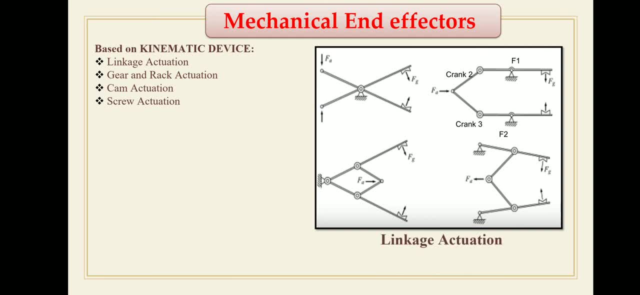 type end effector. a mechanical gripper is an end effector that uses mechanical fingers actuated by mechanism to grasp of an object. okay, shown in this figure. so mechanical figure or mechanical fingers, the primary reason to use mechanical finger. mechanical fingers are generally used to grasp the object, so 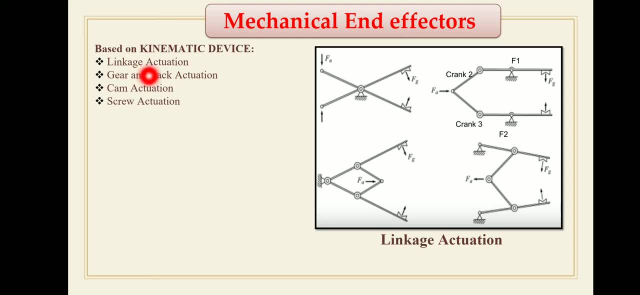 these are the different types of mechanical fingers or mechanical end effector, accord, or based on the kinematic devices. so first device is our first type of mechanical devices. linkage actuation, okay, different types of linkage actuation according to linkage actuation. then, second, use of gear or rack. 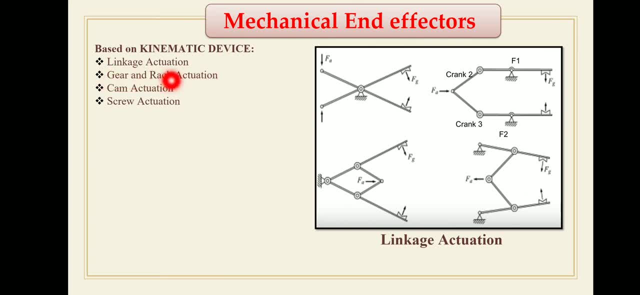 and pinion arrangement, or rack and pinion actuation. then third is the cam actuation, okay, use of cam and follower for actuation purpose. and fourth one is the screw actuation. so in this particularly first type of mechanical end effector, linkage actuation or linkage actuation, so mechanical grippers. 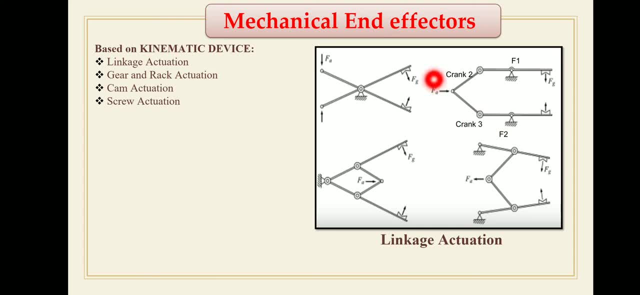 so this figure shows mechanical type end effector: okay. or this whole figure shows linkage actuation. so this is the most popular mechanical gripper for the industrial application- okay. or this device content: pair of slider crank mechanism. slider crank mechanism. pair of slider crank mechanism. so in this particularly linkage. actuation. it consists of two cranks latestели, incase of glyph Brether's in the. so, in this particularly linkage actuation, it consists of two cranks latestley, incase of two cranks latestley, and little bit slightly this slide elastic ought be and of course, 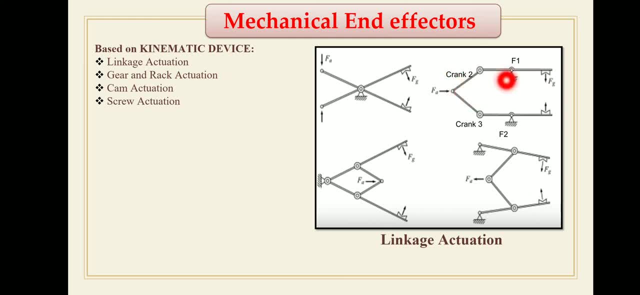 we understood about the daí: someone es Chamob, there's nothing. the post and then dance. CSR should be mentioned. itñaf, 자연ome, that condition of the thriving, such as long run up hetetone busted. crank number first, crank number second. two fulcrums: fulcrum f1, okay, fulcrum f2 and two fingers. 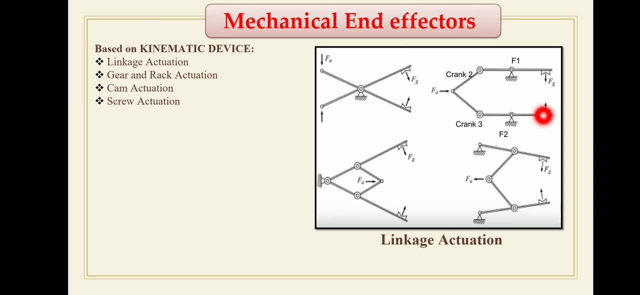 finger number first and finger number second. so in that slider crank mechanism shown in figure, this is the slider crank mechanism. so when piston- okay, or this force or this is the simply pneumatic piston, or piston is pushed by a pneumatic power or pneumatic pressure to the right, when the piston 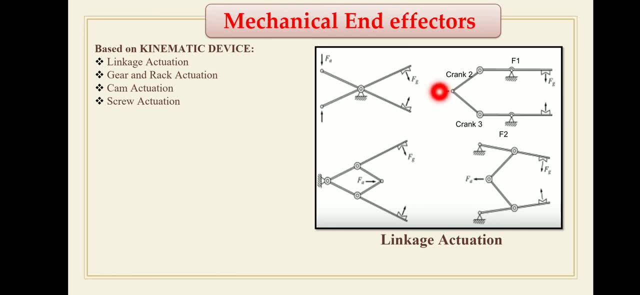 moves from left to right. at the same time, the element in the crank number second and crank number third rotates counterclockwise direction- okay. counterclockwise direction with fulcrum f1 and counterclockwise direction with fulcrum f1- okay. and clockwise direction about fulcrum f1. 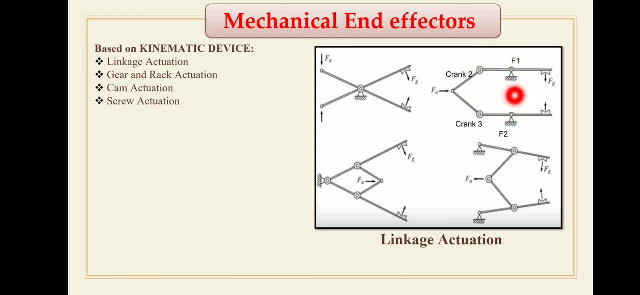 f2. so resulting notation: or it gives or it makes the grasping action at the extended end. okay, it gives the grasping action at the extended end of crank number second and crank number third. the releasing action can be obtained by moving the piston. left to right, means when piston moves from. 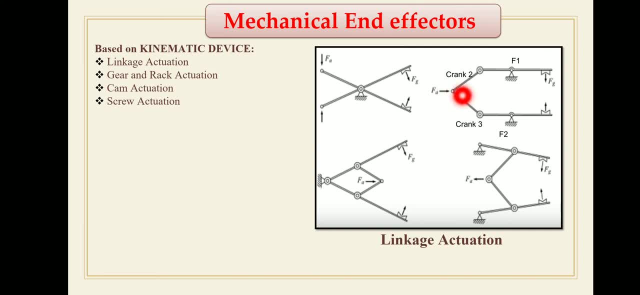 left to right, okay, left to right, the releasing action is taken out. and when piston moves from right to left or a reason, action can be obtained by moving the piston to left means right to left. so this is the simply working principle of slider crank mechanism or mechanical type end effector linkage actuation. mechanical type end effector means in the slider. 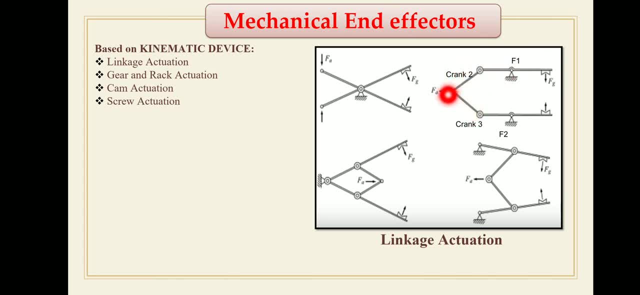 crank mechanism shown in figure. this is the slider crank mechanism shown in figure. this is the slider crank mechanism shown in figure when install, or at the bottom, markibel and the lat Wonderful, how to control the load right of the pump alone, how to control the load at that plate. this could be in any of the following: